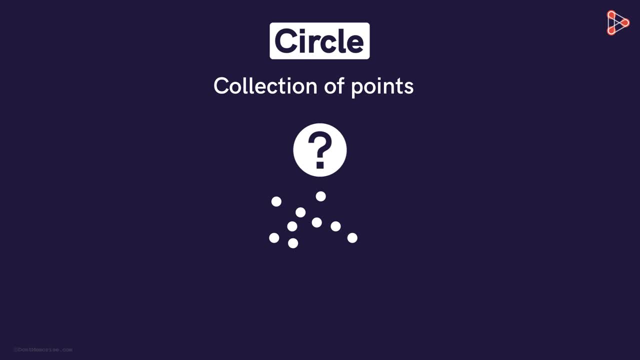 But can randomly placed points form a circle? No, right. So can you tell me how the points come together to form a circle? That's right. A set of points on the same plane which are at an equal distance from a single point form a circle. 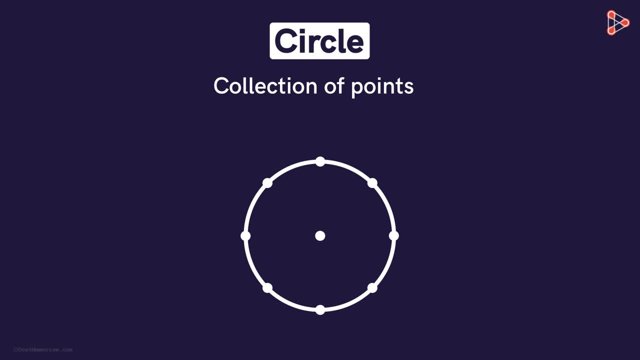 Yes, a set of points on the same plane at an equal distance from one single point. This single point is called the centre of the circle and this distance between the centre and all the points is called the centre of the circle. This is called the radius of the circle. 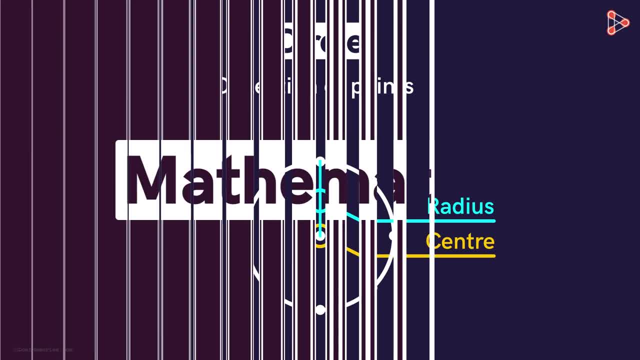 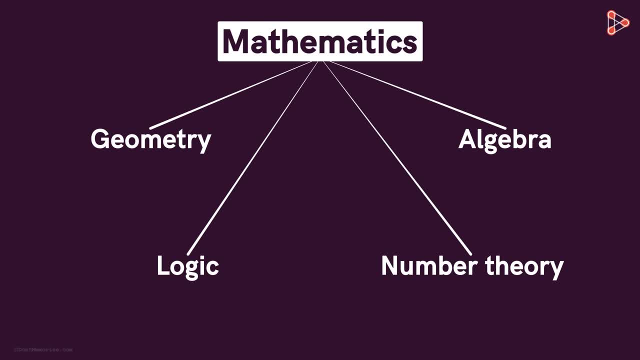 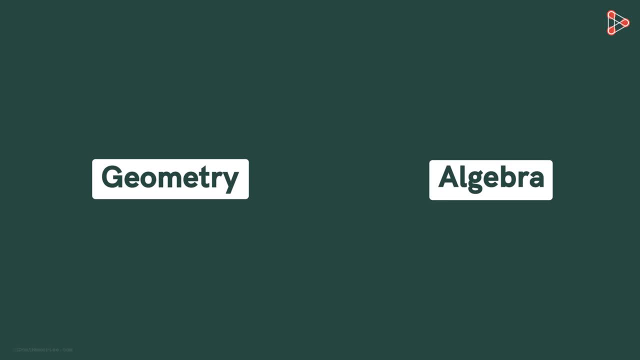 Now let's see something interesting. Mathematics has a lot of branches, such as Geometry, Algebra, Logic, Number Theory, etc. But for now, let's focus on Geometry and Algebra. Let's see how we can represent a circle in Geometry as well as Algebra. 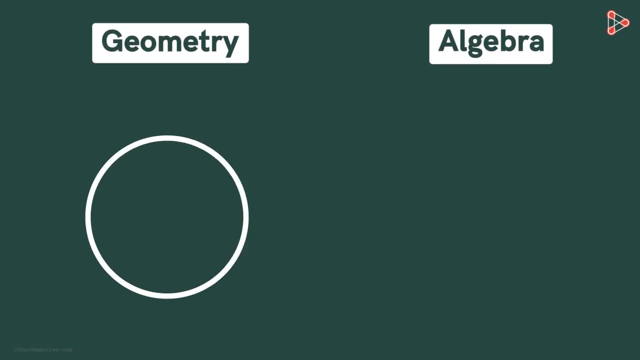 We all know that this is the geometrical representation of a circle, But do you know it's Algebraic representation. So the Algebraic representation of any geometrical figure is called an equation. To find the Algebraic representation of a circle, we need to find its equation. 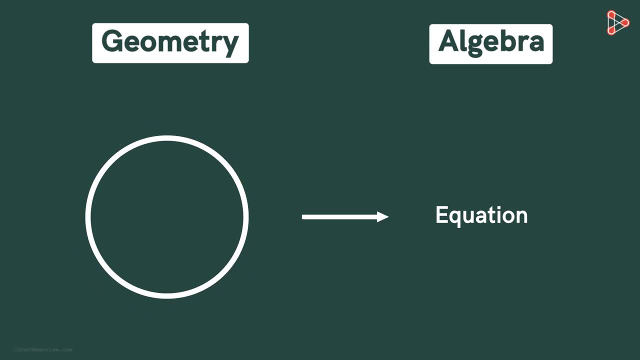 To find the equation of a circle, let's name a few things. Let the centre be O and let its coordinates be H comma K. Similarly, let P be any point on the circle, with X comma Y as its coordinates. Also, let's denote the radius by R. 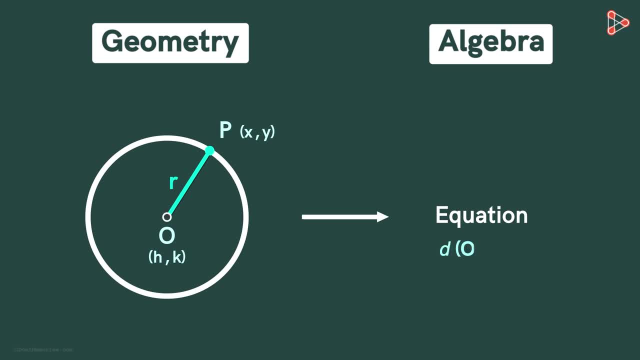 So the distance between points O and P is nothing but the radius. But how do we find the distance between the points O and P? Since we know the coordinates of O and P, we can find the distance OP using the distance equation. So we get this. 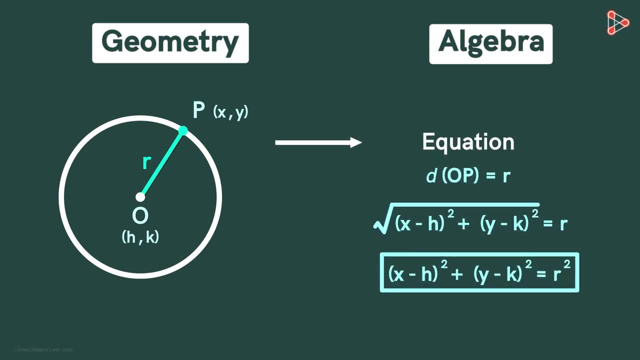 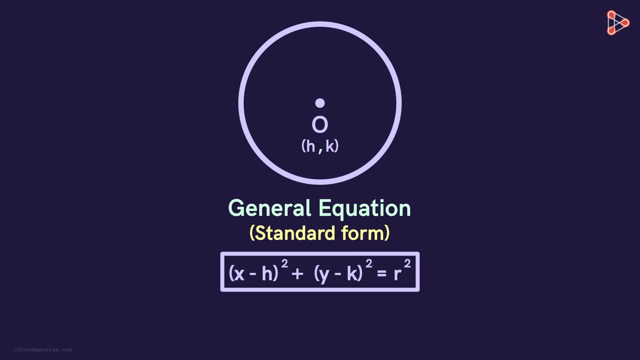 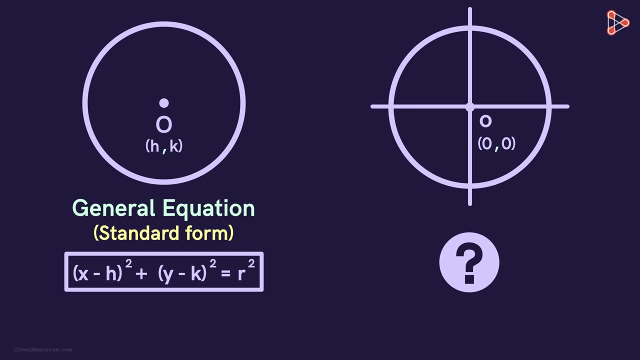 Squaring both the sides, we get this. This is the general equation of the circle. Now that we've seen the general equation of a circle, can you tell me the equation of a circle whose centre lies on the origin? Since the centre is the origin, the values of H and K become zero.